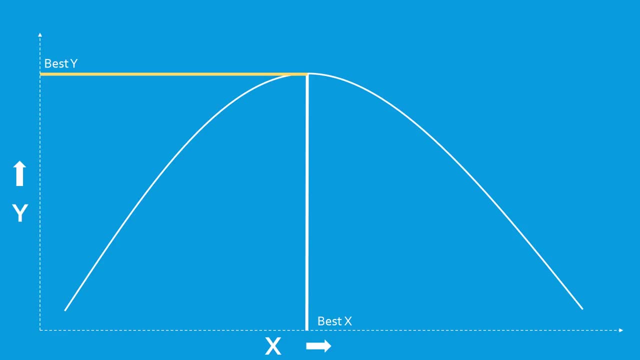 Guessing and checking can take much too long, and it can be difficult to find the values where the derivative is equal to zero. To find the answers to most optimization problems, we need to use a special type of program called an optimization algorithm. We'll talk more about optimization algorithms in upcoming 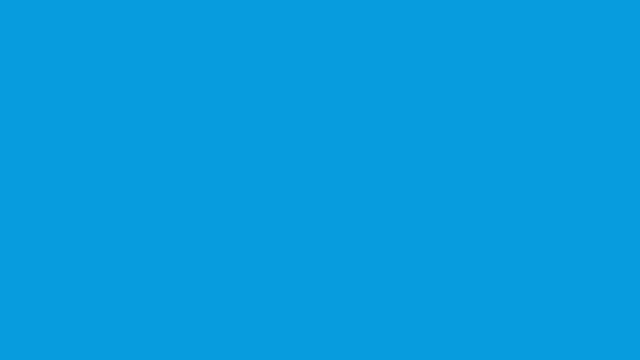 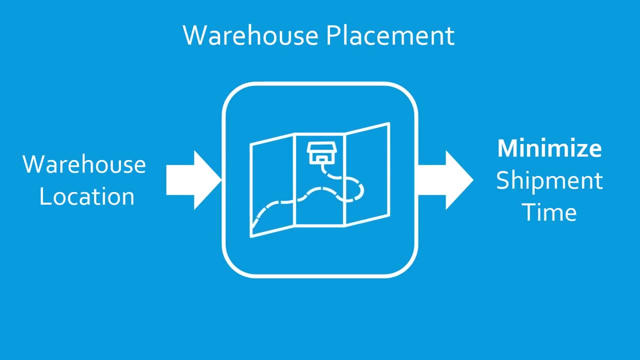 videos. Optimization can be applied to a huge variety of situations and problems. For example, choosing the optimal location for a warehouse to minimize shipment times to potential customers. designing a bridge that can carry the maximum load possible for a given cost. choosing the optimal build order for units in a strategy game to amass the strongest army possible. 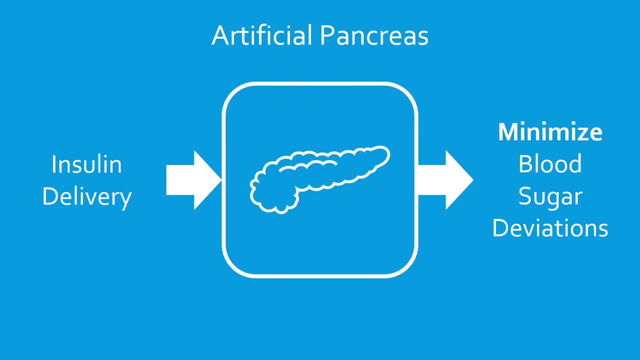 in a given time. controlling the insulin output from an artificial pancreas to minimize the difference between actual and desired blood sugar levels throughout the day. designing an airplane wing to minimize weight while maintaining strength. selecting the best set of stocks to invest in to maximize returns based on predicted performance. 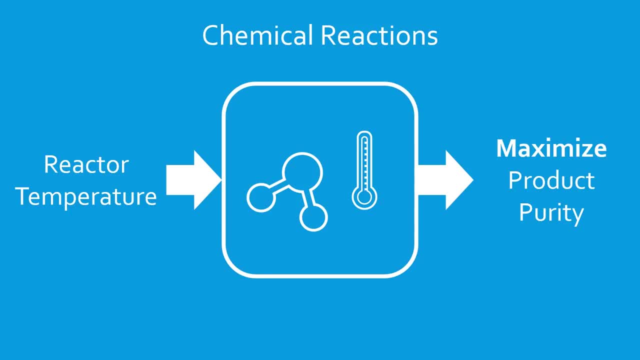 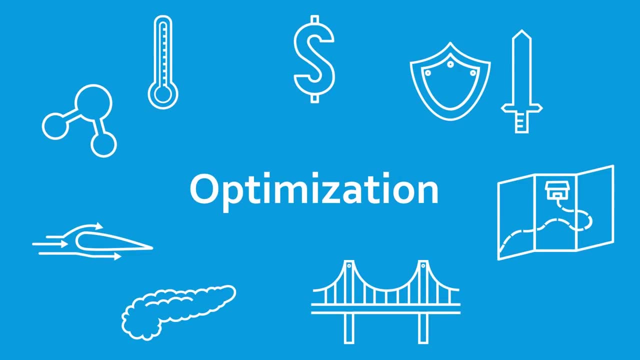 controlling the temperature of a chemical reaction throughout a process to maximize the purity of a desired product. As you can see, optimization is a powerful tool in many applications. This is just a small sampling of the many fields that make use of optimization techniques to improve the quality of their solutions. If something can be modeled mathematically, 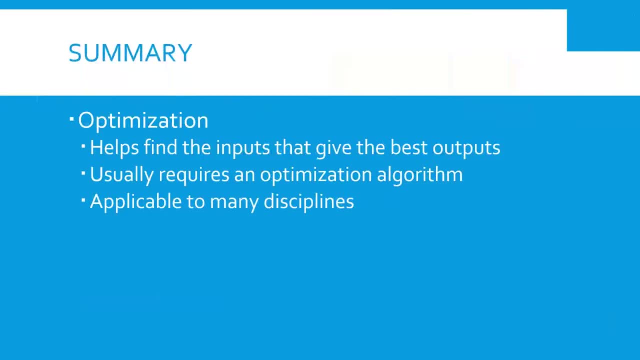 it can usually be optimized. To summarize: optimization improves results by helping to improve the quality of the product, By helping to choose inputs that produce the best outputs. Most optimization problems require an optimization algorithm to solve, And optimization is applicable to many disciplines. 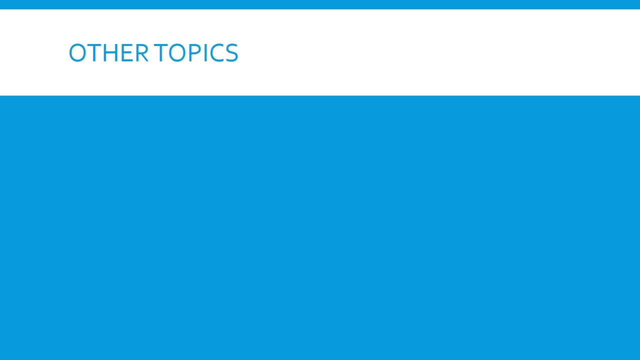 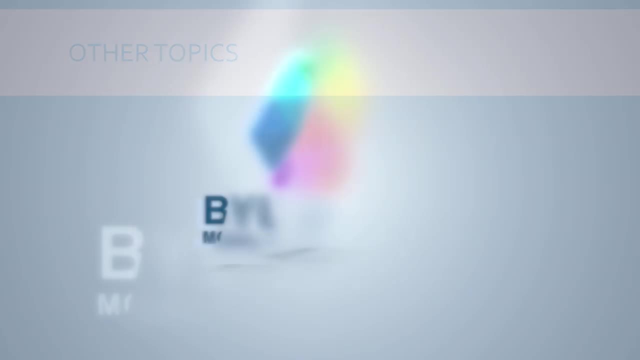 Thank you for watching. I hope you've enjoyed the video. Follow these links to see more videos on other optimization topics. I'll see you in the next video.